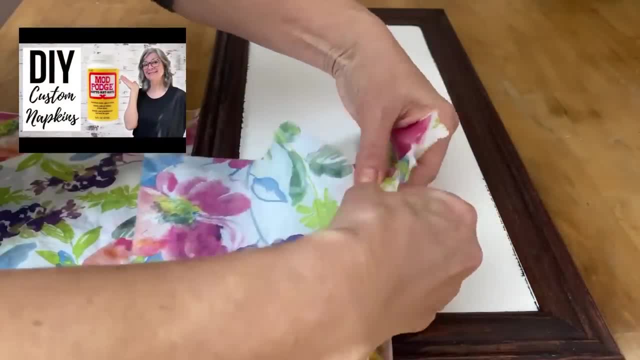 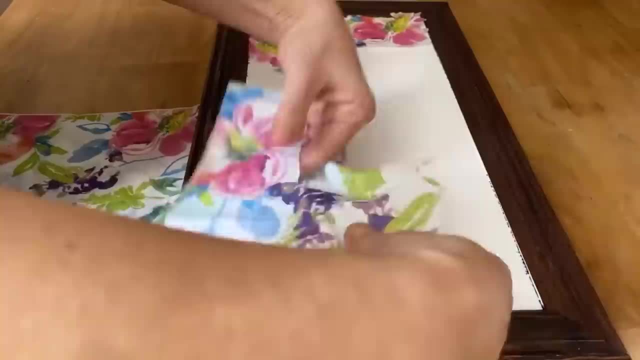 front two plies. Don't throw them out. I saved them for another project, but we're going to just use this one ply that has the flowers on it. I like to tear my napkin around the edges When you're decoupaging. it just helps it blend in better on your project. And I'm just tearing. 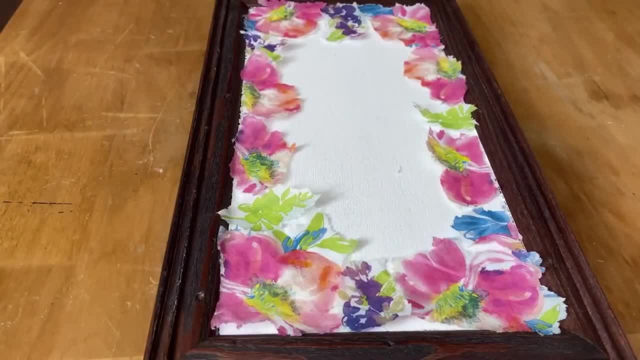 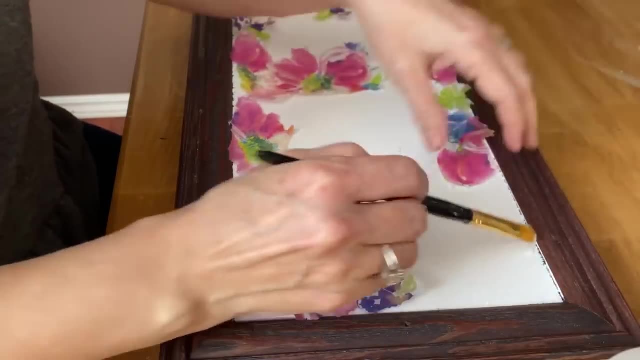 around these big floral pieces and piecing it around my frame until I like the way that it looks. I'm going to be using my Mod Podge mat. You can use any decoupage product. I prefer this one. It works the best for me and you can also use a mat. 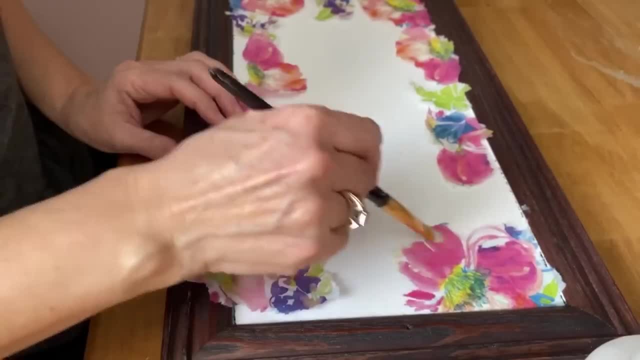 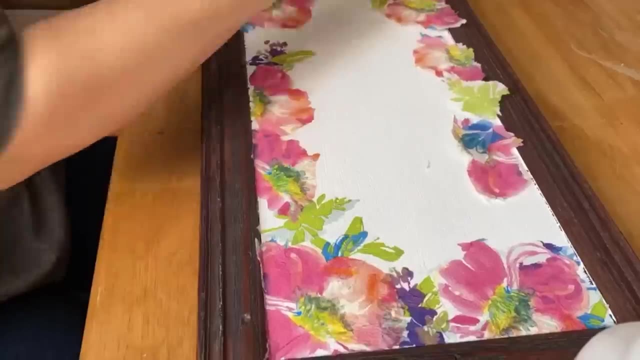 Or a glossy, depending on what you're looking for when you're completing your project. I'm just putting a light coat of Mod Podge underneath the area where the napkin is going to be, and then just another really light coat on top of it to secure it all in place. We're not going. 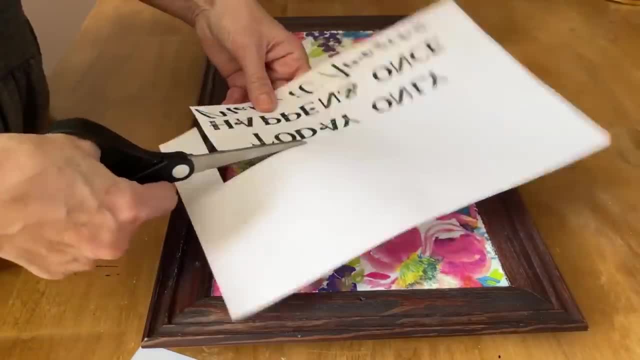 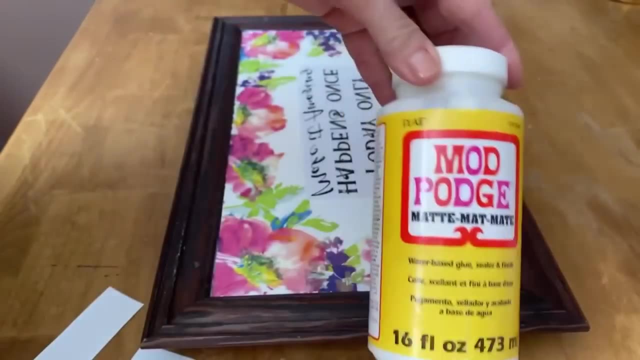 to worry about the little bits overhanging right now. We can clean that up when it's all finished. I've decoupaged my napkins all around the outside so it looks a bit like a border and I'm going to put a quote in the middle. I'm going to do my Mod Podge reverse graphic transfer method. I've 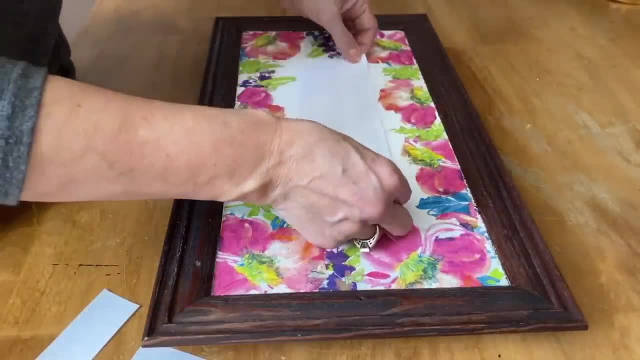 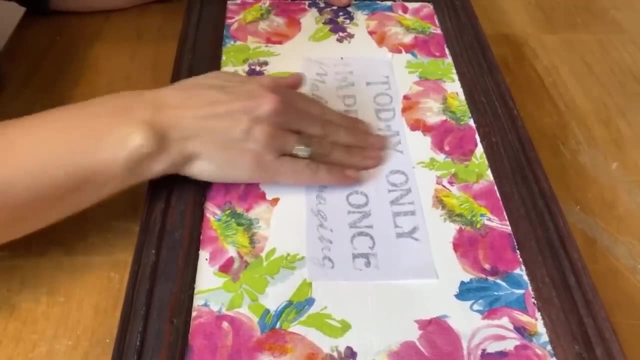 printed this off on my laser jet printer, made sure to reverse the text and I'm going to center it right where I want it. Let it dry completely overnight, 24 hours, and then, when it's dried, we're going to dampen it with a little bit of water, rub away the paper and we're going to 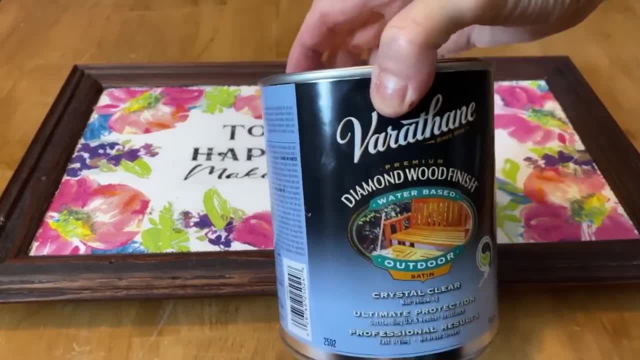 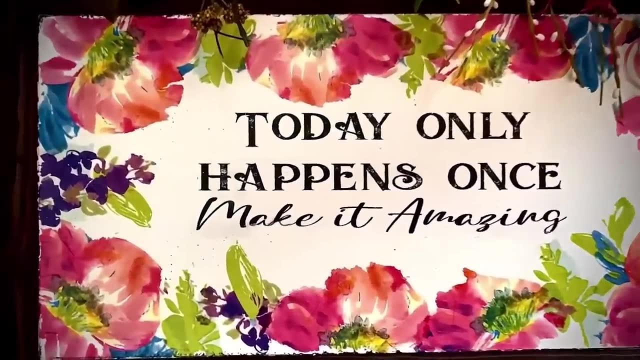 have a beautiful graphic on our project. I'm going to seal it all up with a poly acrylic sealer. You don't want to put much on, just a really light coat. If you apply too much of a top coat it will bubble up on you. I prefer the poly acrylic sealer as a top coat over the Mod Podge. 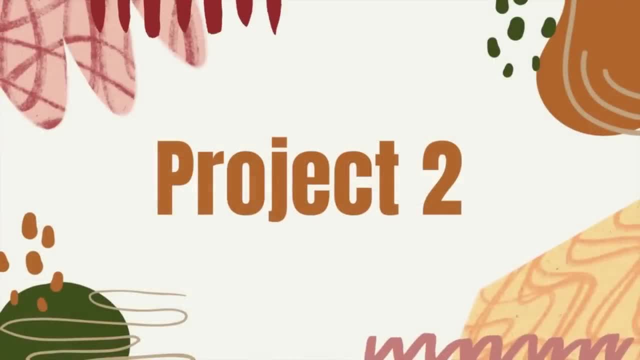 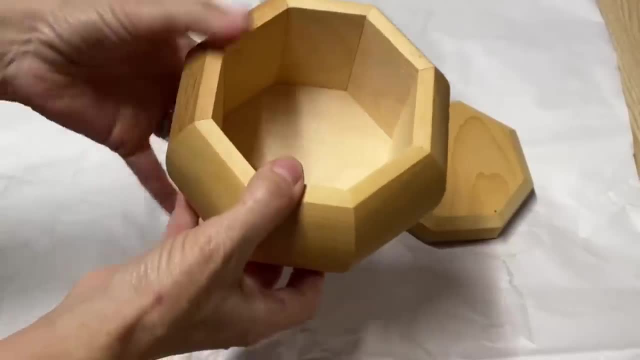 And there you have a beautiful canvas and upcycled frame. Next decoupage project that we're going to work on is this bowl that I found at the thrift store. It's beautiful and I love that it has a lid, And I have the perfect napkin that I want to. 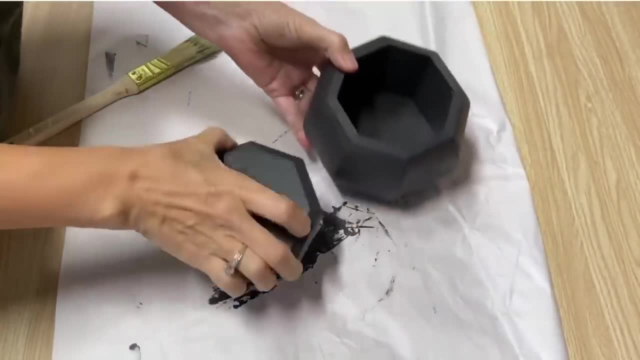 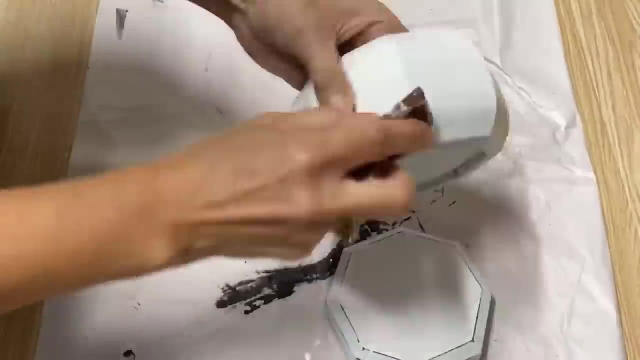 decoupage with. I'm going to give this a bit of a distressed look when it's all finished. So I've painted my base coat with my black chalk paint. When that was all dry, I put on a coat of my white chalk paint because when we sand we want that. 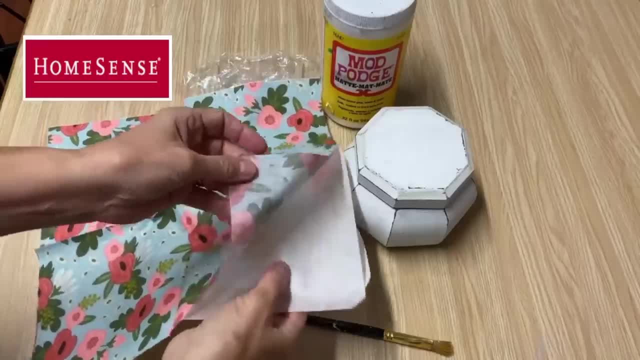 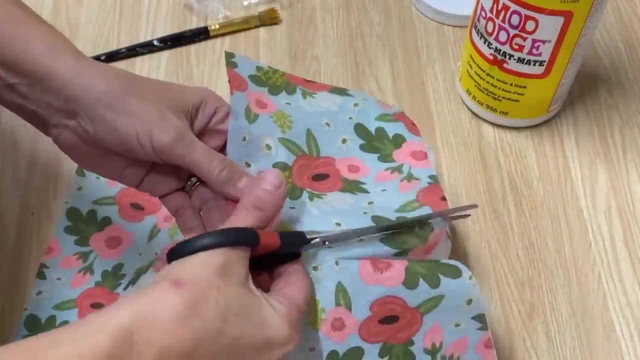 black to peek through a little bit. I picked these napkins up at HomeSense. Absolutely love them. It's going to be perfect for this little project Because this little container has so many sides. we're going to do it in stages. 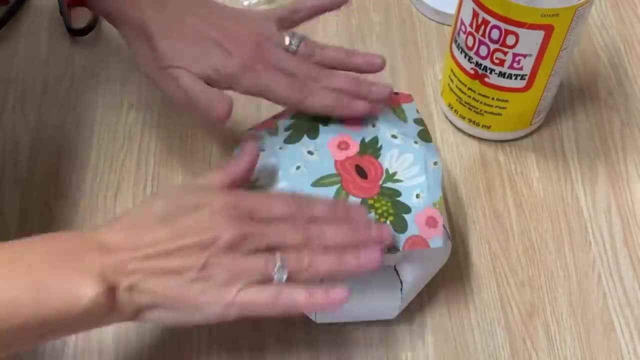 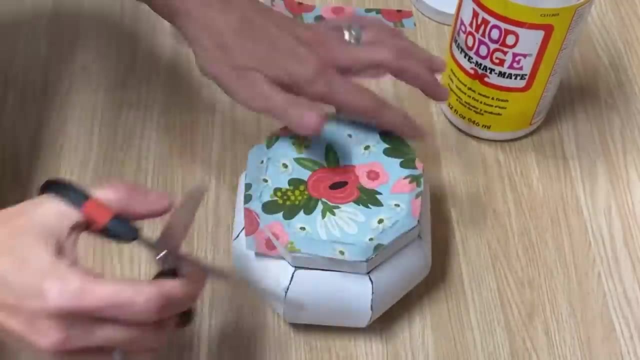 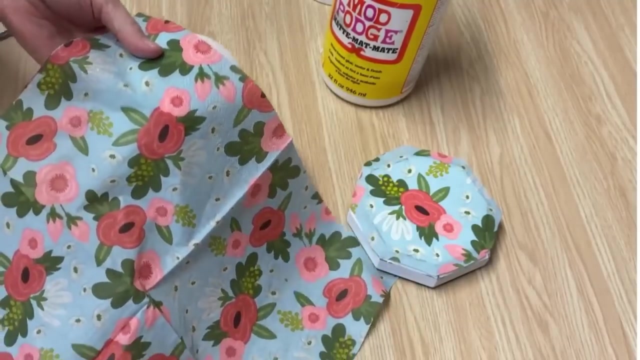 I'm going to do the panel on the top first, making sure I've cut out my napkin so I have the floral image that I want in the middle of it. Trim off the extra, then we're going to set it aside and let it dry, And then for the side panels, I'm going to do every other panel If we try to decoupage. 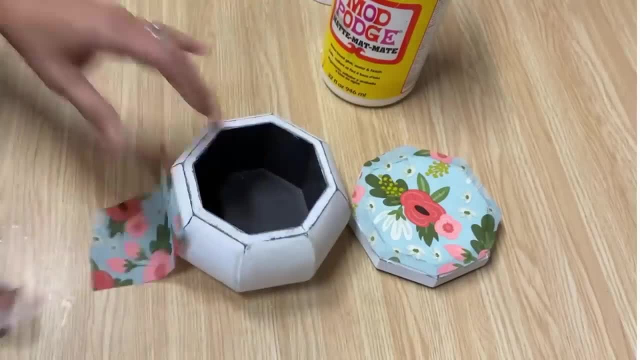 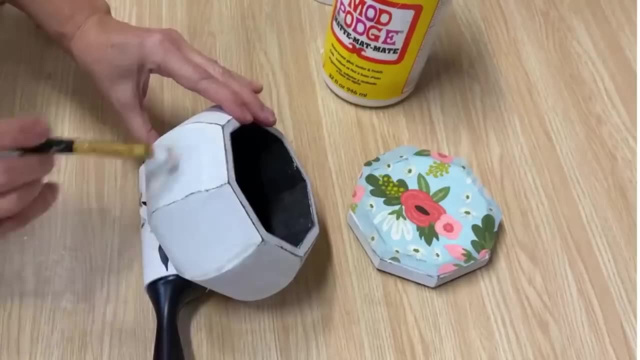 this napkin all in one piece, it's going to be miserable. it will be full of wrinkles and full of bubbles. so if we just do this in separate panels, it will go on a lot smoother and a lot easier. cut out your napkin a little bit bigger than the panel. place it down with a little bit. 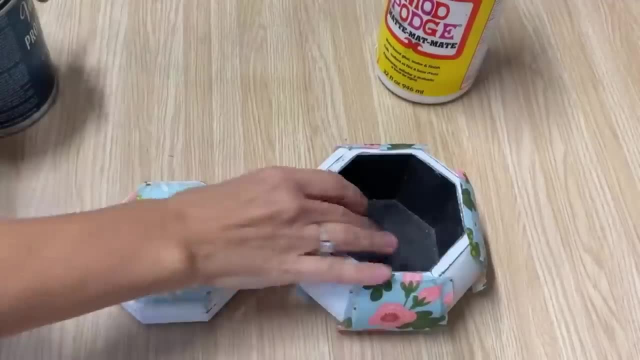 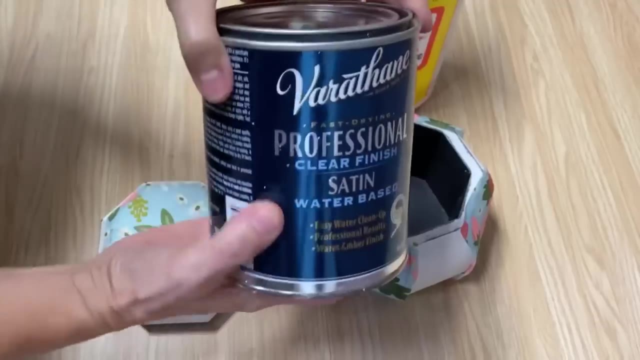 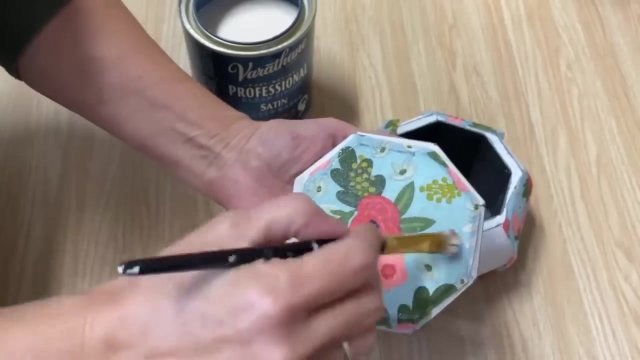 of mod podge and then i like to use some saran wrap or cling wrap. it just helps get rid of the wrinkles and bubbles without tearing the napkin. once i had every other panel done, i set it aside and let it dry completely. now i'm going to put on the poly acrylic sealer now, on all of those dried. 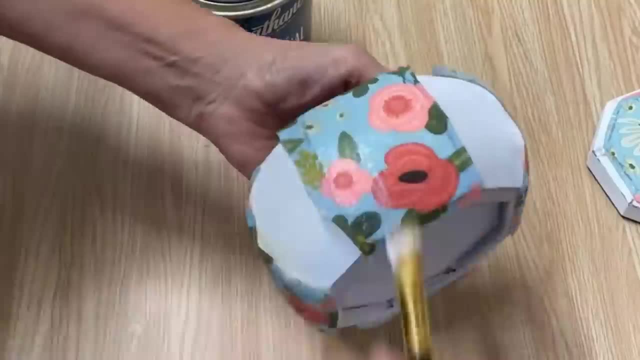 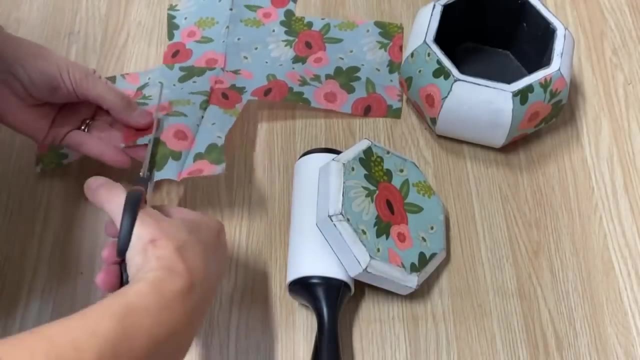 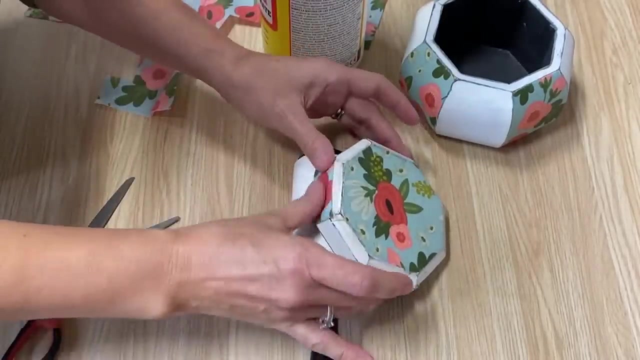 pieces- all those panels and the top, set it aside and let that dry. once everything's completely dried, i'm taking a 220 grit sandpaper and i'm sanding off all the extra bits of the napkin around the sides. we're now ready to go on to some other panels. same thing we're going to. 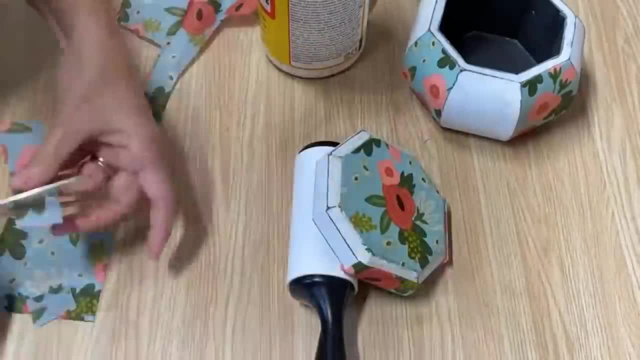 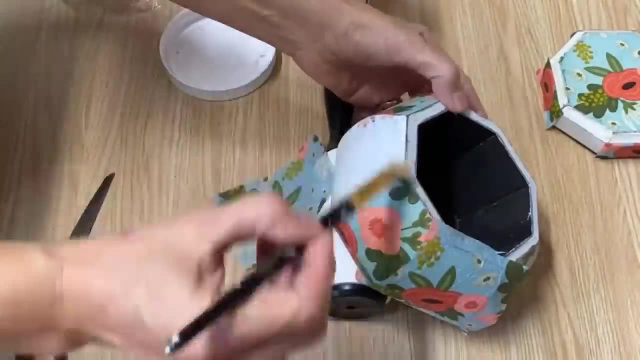 do every other panel. use some saran wrap, get it nice and smooth, set it aside and let it dry completely. i know this is really time consuming, but when you're all finished, you'll be much happier with your project, without having any bubbles and wrinkles and trying to work with. 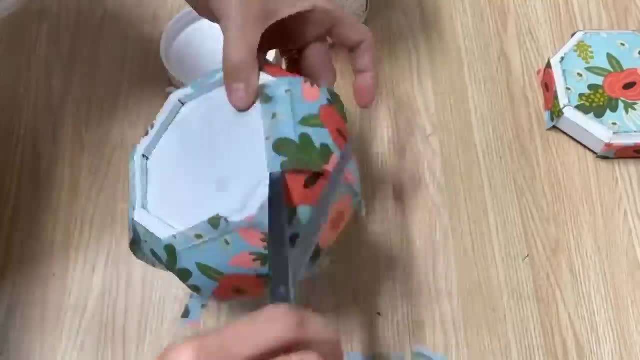 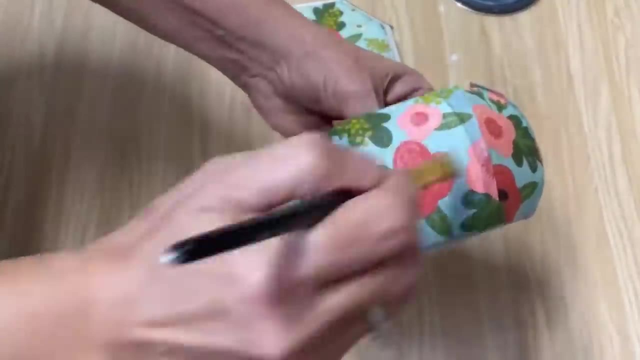 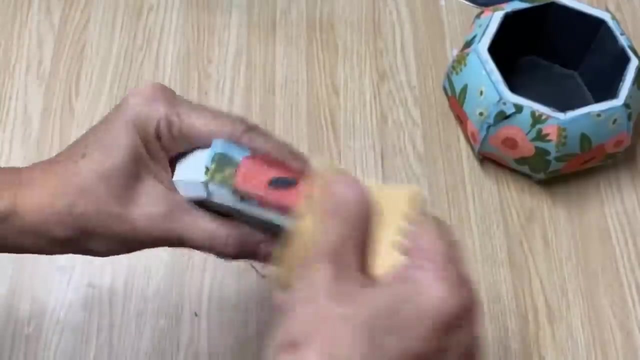 a full napkin. whenever i go to the thrift store, i always keep my eye out for little bowls or dishes or plates or anything that i can upcycle and make pretty again, especially if it's dated. there's so many beautiful napkins that you can choose from that will make your project just pop and again. 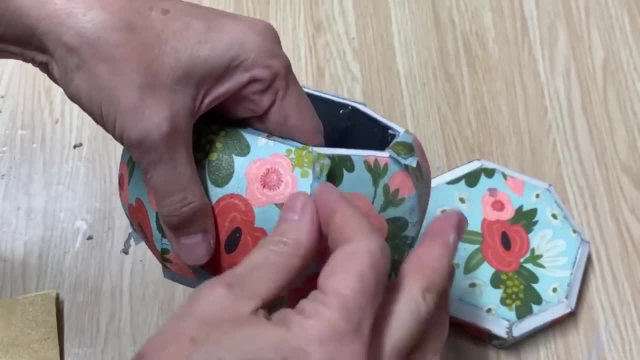 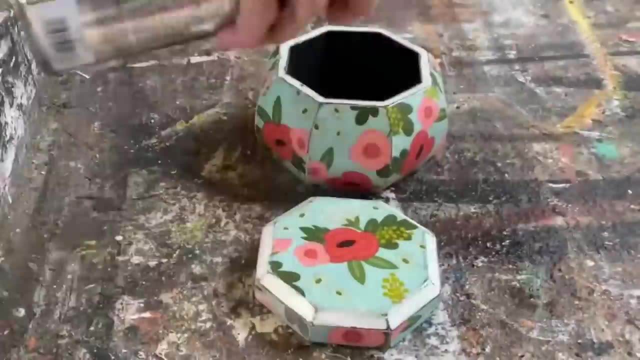 everything's dry. i take that 220 grit sandpaper and you can see how it just makes a nice crisp line when you sand it. now i'm going to be using this little container quite a bit, so i want to seal it up with an engine. enamel makes it really durable. i let that dry completely and then i 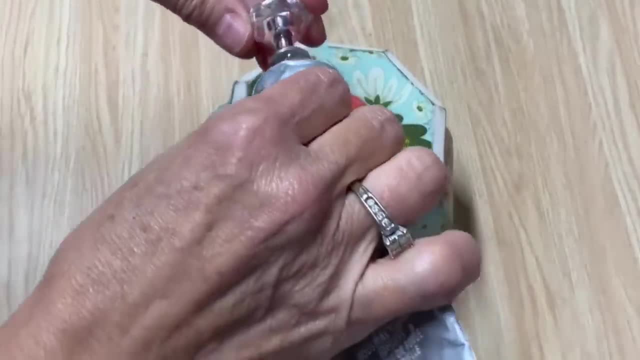 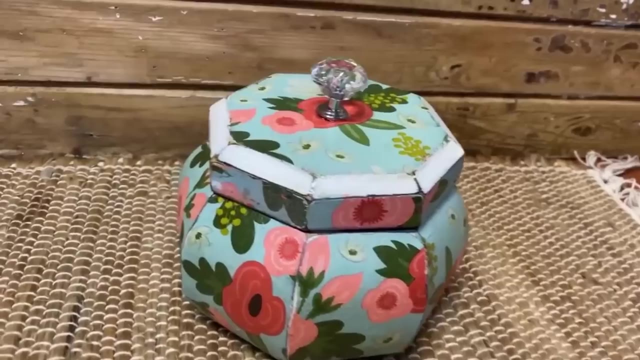 thought it needed a nice little knob on the top. using my e6000, i had this little glass knob and i'm going to glue it right to the top of that. finished it off beautifully. so there we have a cute little container i'm going to keep my earrings and rings in. 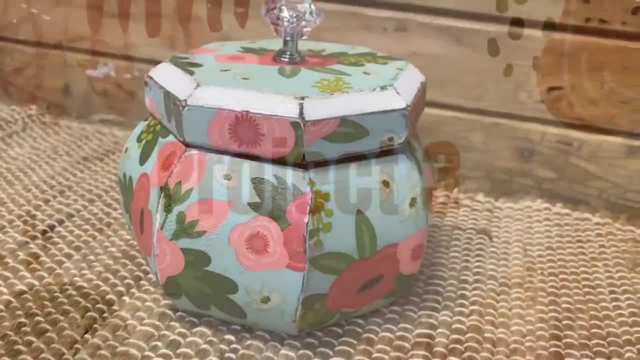 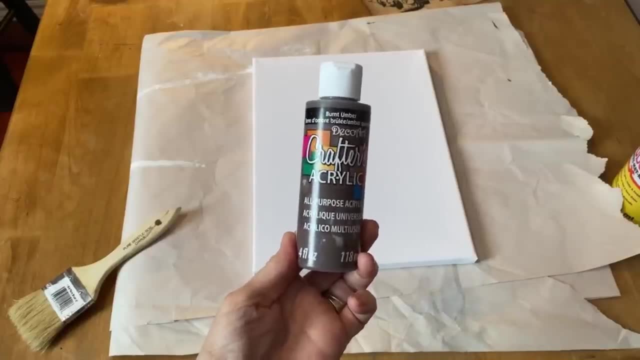 with a thrift store find that i've decoupaged with a beautiful napkin. next project is also a really easy one for the beginner. i bought this artist canvas at the dollar store and we're going to use our acrylic paint after that acrylic paint has completely dried. 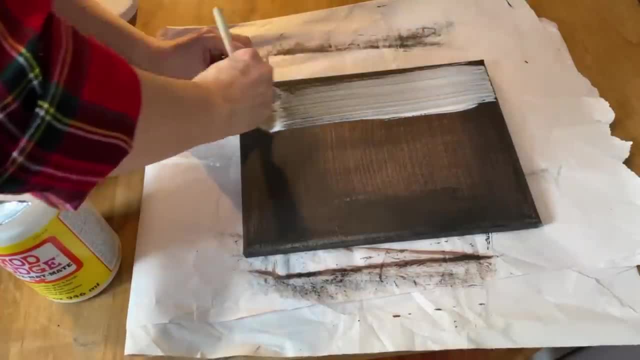 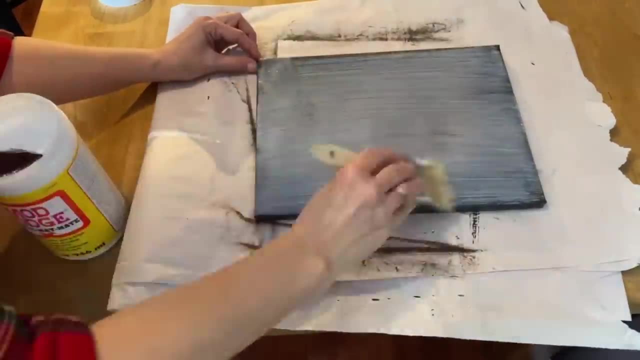 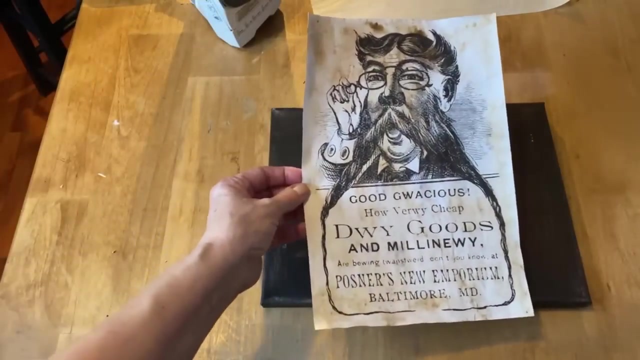 i'm going to put on a really thick coat of the matte mod podge. i'm going to show you, with this project, how easy it is to decoupage, doing the iron-on technique. after the first layer of mud completely dry, we're going to reapply a second coat and let it dry completely after that second. 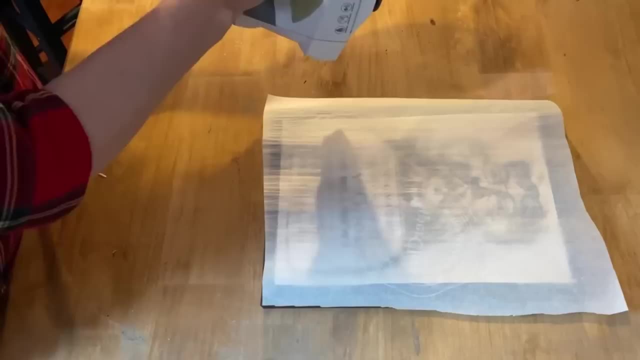 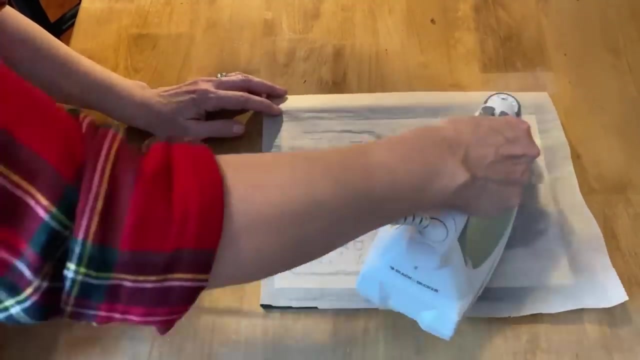 coat has completely dried, i have printed off this graphic from the graphic fairy and we are going to lay it on top of that canvas and then put a piece of parchment paper over top of it, and then we're going to iron on the highest setting with no steam. 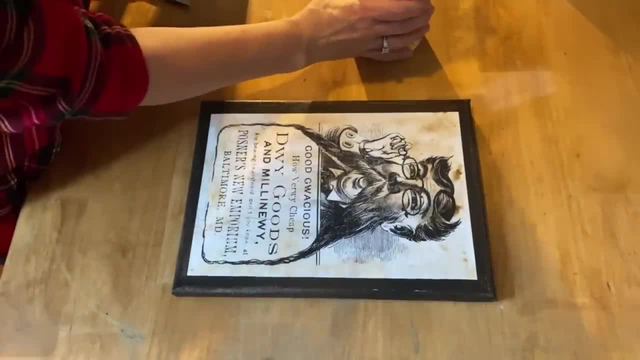 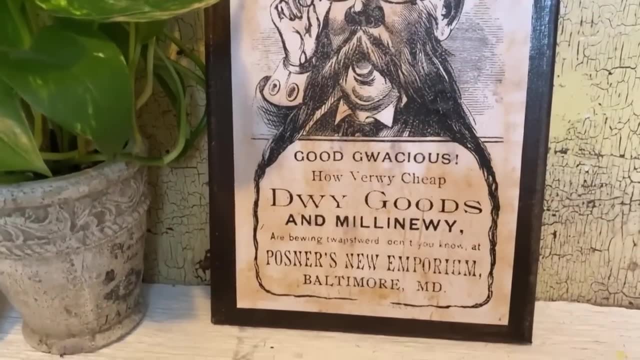 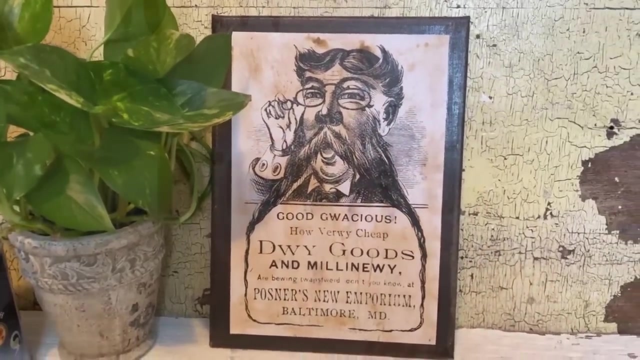 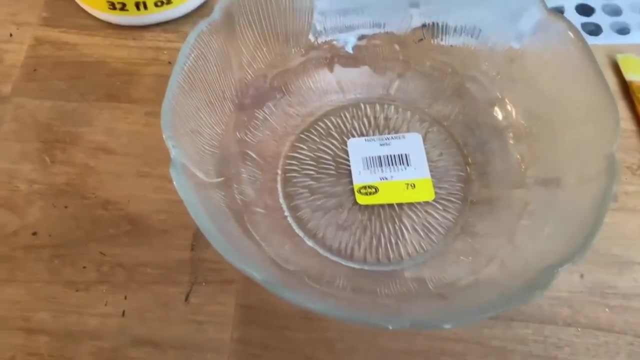 and that paper is going to melt right into that mod podge and adhere it. simple, easy way to decoupage: i'm putting a really light coat of the mod podge on top to seal it up and we have this beautiful graphic on a canvas. i've got so much decoupage information in here. i hope i'm not overloading you, but these 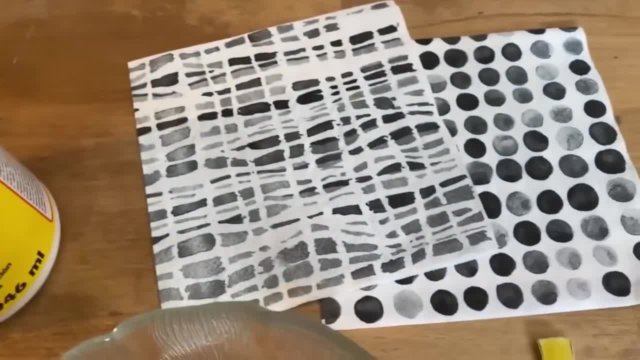 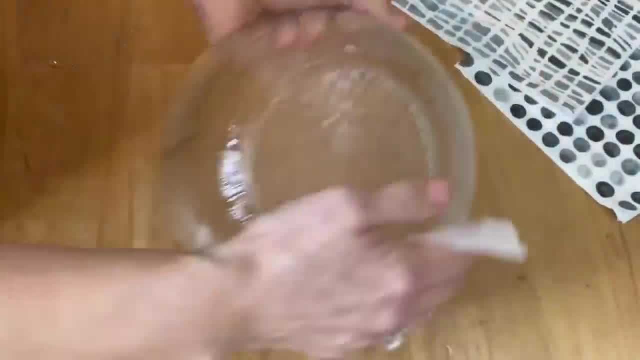 are all so fun. i wanted to share them all with you. the next project we're doing is this glass bowl, and this is fantastic. we are going to use two different napkins with this project and, before we start, we want to make sure that we have the right amount of decoupage, so we're going to put 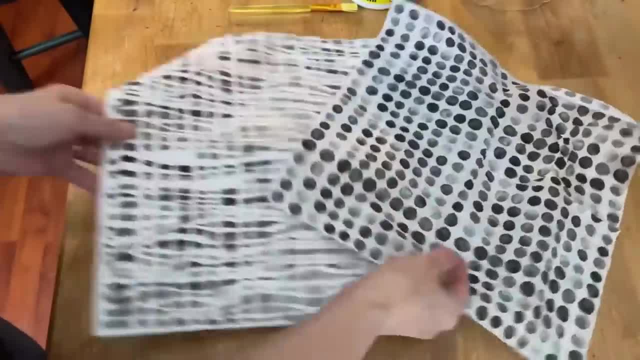 a piece of parchment paper on top of it, and then we're going to lay it on top of it, and then we're going to lay it on top of it, and then we're going to lay it on top of it, and then we're going to. 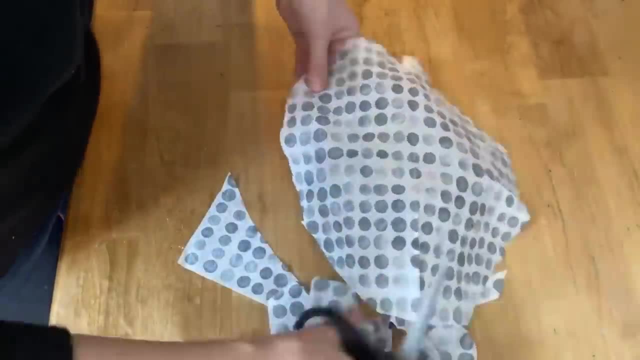 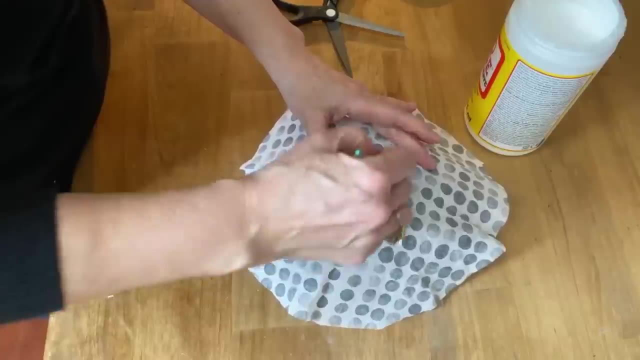 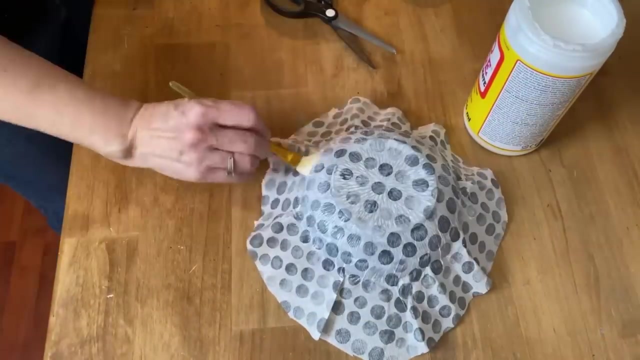 use one ply of these napkins. the first napkin i'm going to cut in a circle so it's a little bit bigger than our bowl. i'm going to lay it so the good side is facing in towards the bowl, and then we're going to just start applying our mod podge, starting in the middle and working our way down. 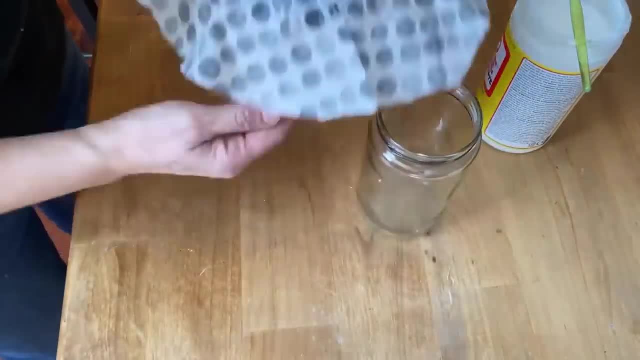 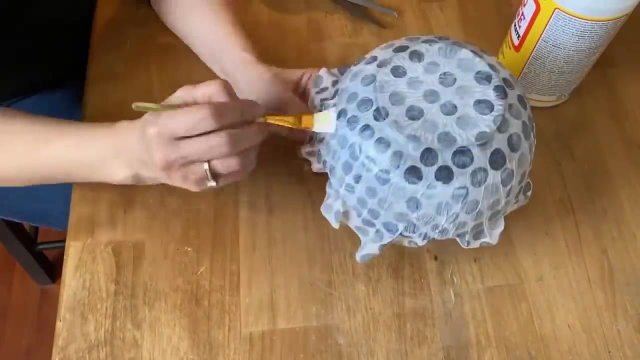 now you are going to get some wrinkles when you're doing this technique because the napkin is not going to completely form smooth around the curves of the bowl. but we're embracing it with this project because it works and it looks excellent. you want to set it aside and 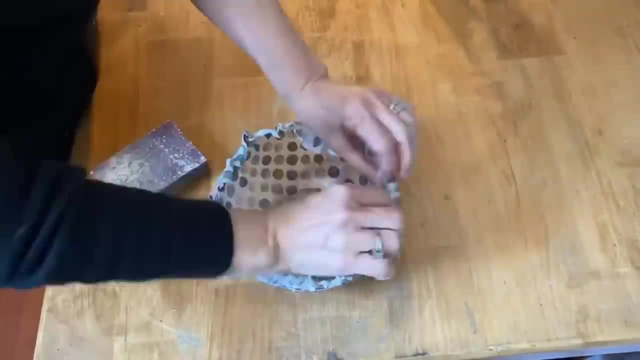 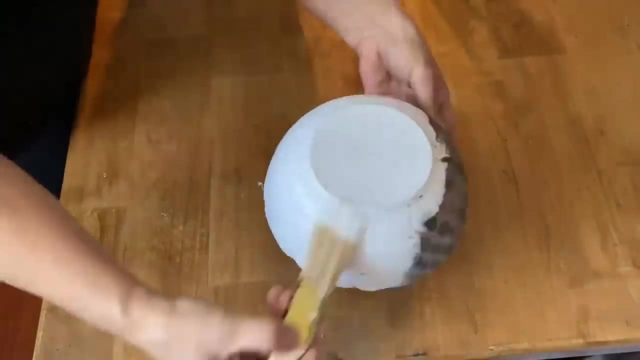 let it dry completely, and then, when it's dry, i'm going to use a sanding block and just remove all the napkin along the top. now comes the magic, so we can see one napkin on the inside and the other napkin on the outside. i'm applying a coat of my homemade white chalk paint. 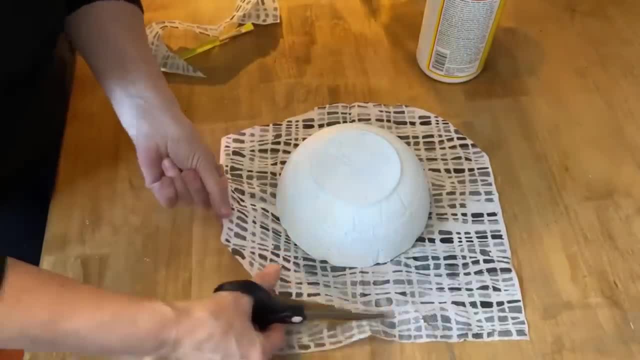 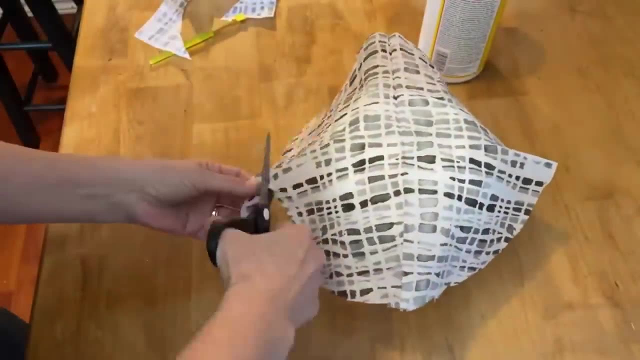 if you don't do this, you will be able to see the other napkin through this napkin because it dries translucent when we're putting the paint on. it will show one napkin on the inside and this napkin on the outside. we're doing this exactly like how we did the first step: start in the middle of the. 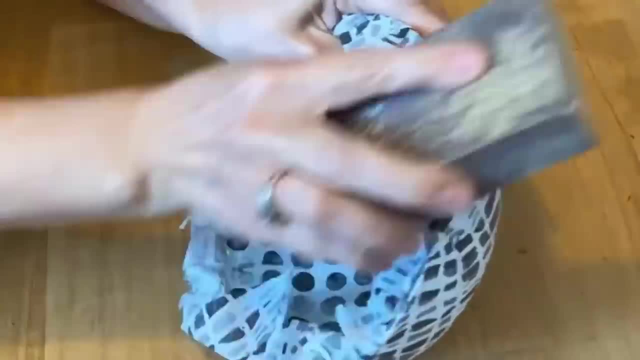 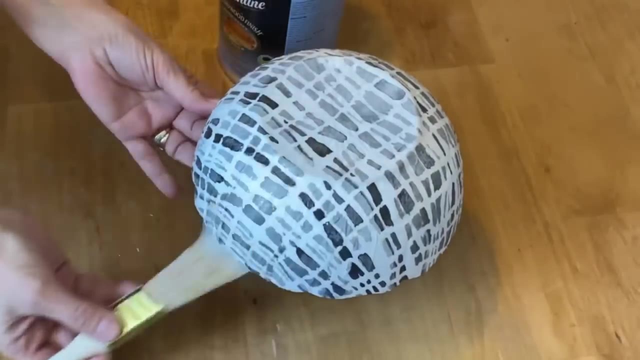 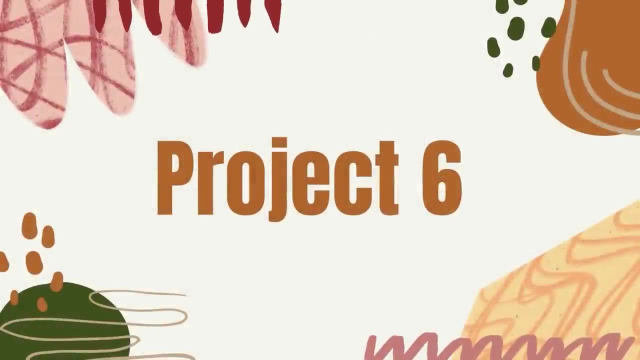 bowl and work your way down, applying mod podge, nice and even, as we go. we've let that completely dry, sand it off the edges and i'm going to seal this all up with some poly acrylic sealer. and how gorgeous is this bowl? simple and easy. next, simple decoupage project i'm going to show you. 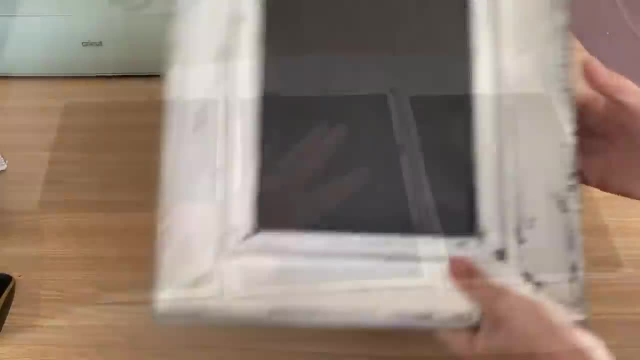 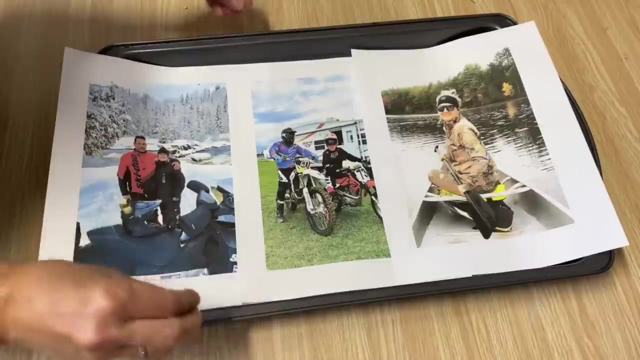 how you can decoupage a picture right into a frame. i've taken the wood out of the back of each frame and i'm going to paint it with some white chalk paint. i'm going to show you how you can decoupage using an inkjet printer. i've printed off some adventure pictures of my husband and i. 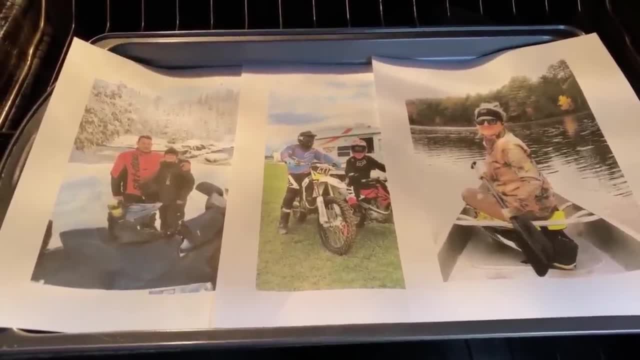 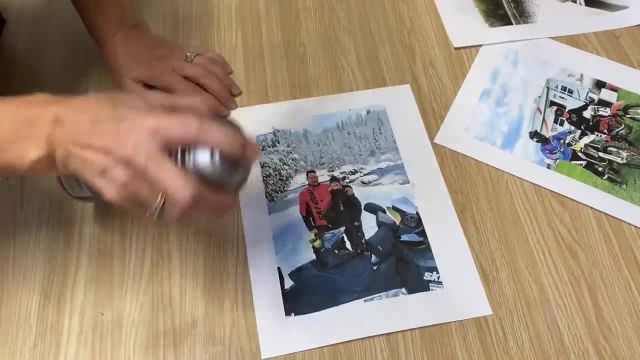 and i've printed these off on my inkjet printer on regular computer paper. i'll put it in the oven for about 10 minutes on the lowest setting and then i'm going to seal them all with some hairspray. if you don't do this step, when you're using an inkjet printer, when you introduce the 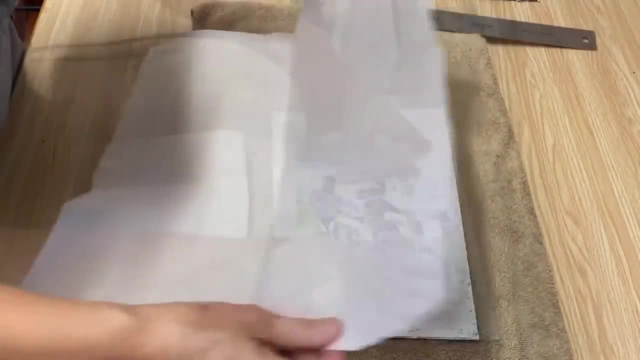 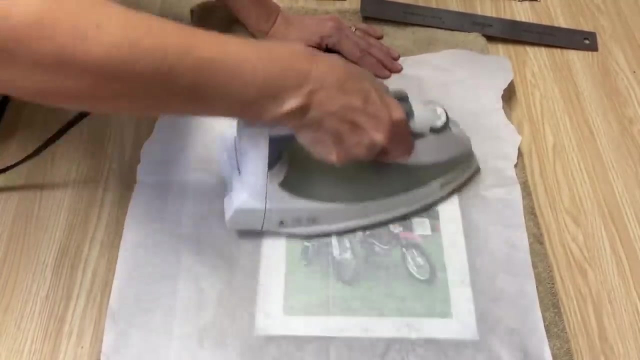 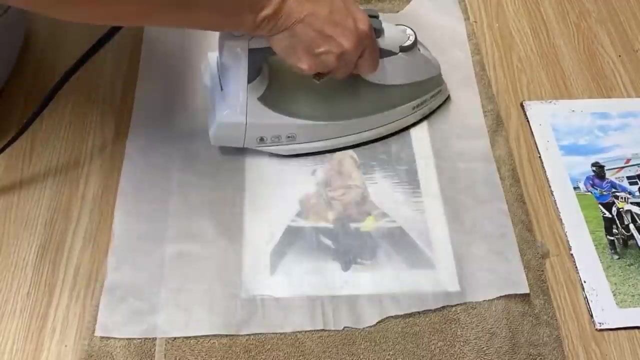 mod podge. the ink may smear or rub off. i've applied two coats of the mod podge, letting it completely dry. in between each coat laid my photo into it: parchment paper, iron on the lowest setting with no steam, and we're ironing it right onto that wood. when you introduce the heat into the mod podge, it. 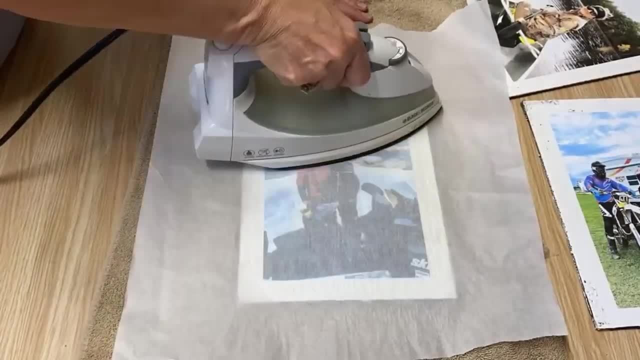 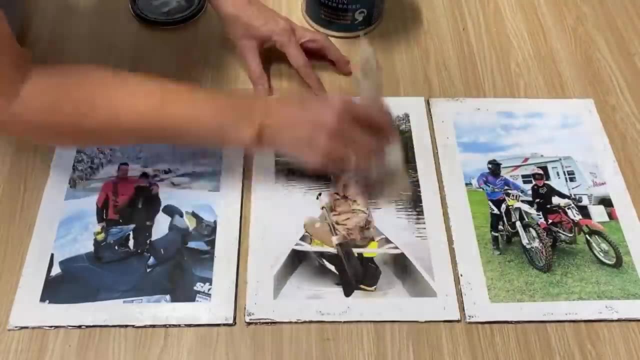 soaks into the paper and it will seal it right on decoupaging it onto your project. i've let everything cool down. now we're going to seal it up with a little tiny bit of the polyacrylic sealer. don't introduce too much or it will bubble and wrinkle again. you just need a really light coat. 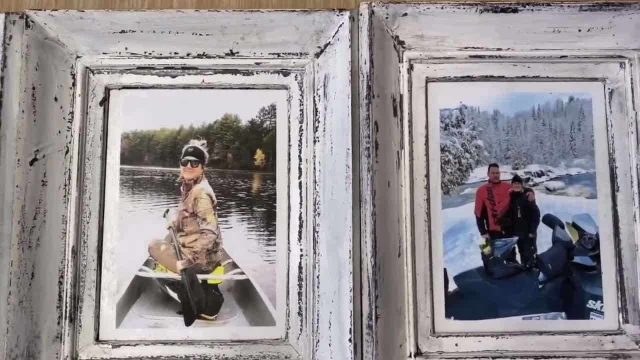 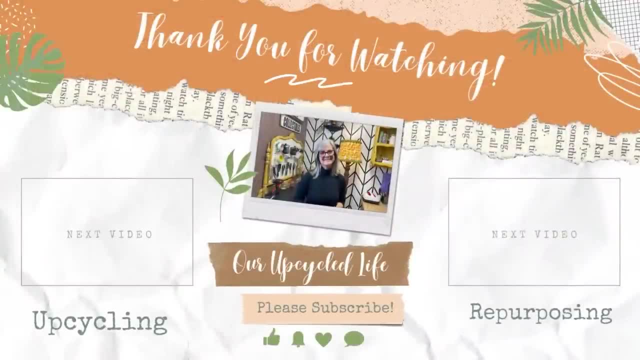 so i hope these projects have given you lots of inspiration to start decoupaging. if you've enjoyed today's video, i'd love for you to like and subscribe and follow along, and if you enjoyed this video, i'm sure you'll enjoy either of these videos and i'll see you in the next one. bye, bye. 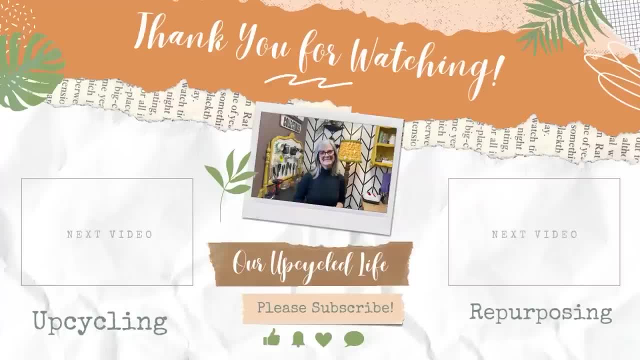 videos. thanks for watching. have a great day and we'll see you in the next video. take care. 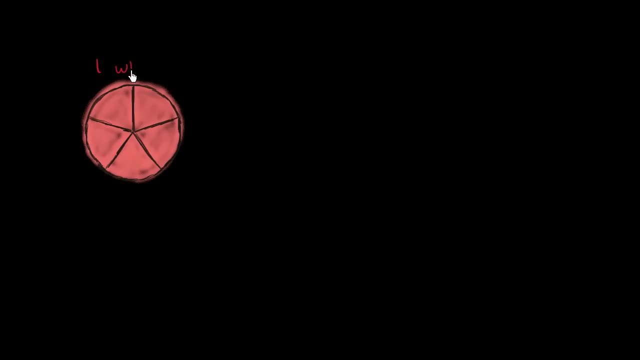 Let's say that this circle right over here represents one, one whole, And we've divided this circle into one, two, three, four, five equal sections. So each of these sections represents one-fifth. Each of these sections represents one-fifth of the circle. 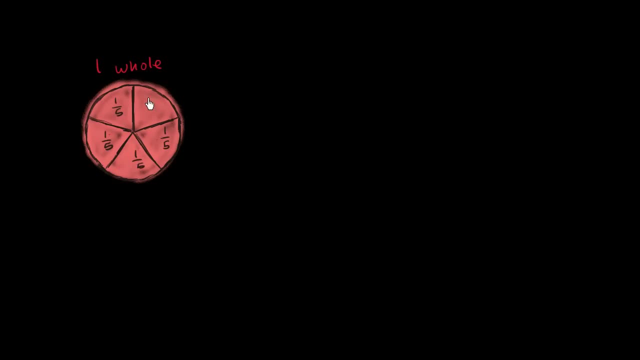 We've seen this already One-fifth, one-fifth, one-fifth and one-fifth. And if we were to then color in some of this? so let's say we were coloring three of these sections, So that's one of the sections right over there. 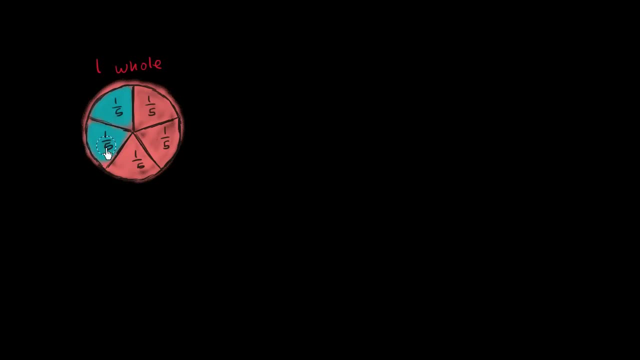 another one right over here. So we've colored in two of the fifths and then three of the fifths. Notice you put those three one-fifths together. how much have we now shaded in? We've shaded in three-fifths of the whole. 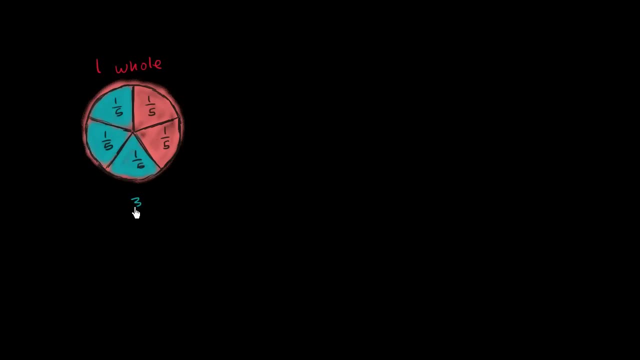 So the fraction that's actually shaded in now is three-fifths. Three-fifths is what's shaded in Now. let's do this. Let's do something in some ways a little bit simpler, but also in some ways, kind of interesting. 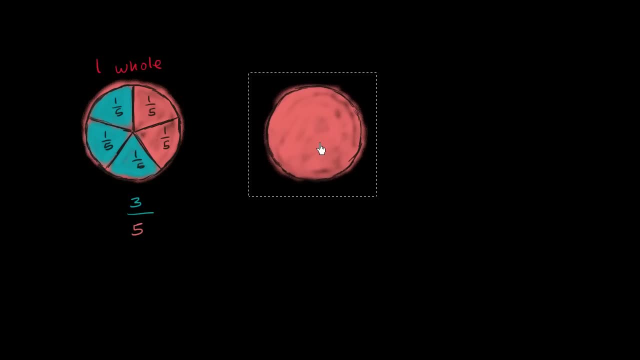 Let's start with a hole again. So, once again, this is one hole. Let me label it one hole. So it's one hole, And instead of dividing it into five equal sections, I'm just going to divide it into one equal section.